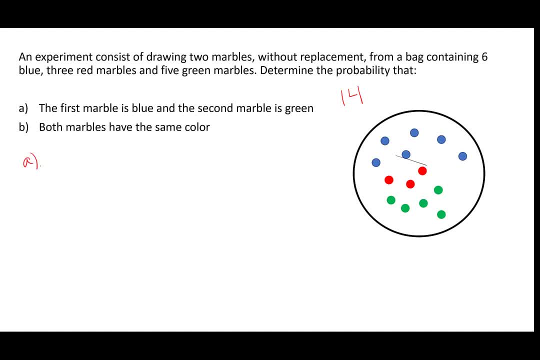 So part A, the probability that it would be blue is six fourteenths. Then the probability that it would be green After one marble is removed is five thirteenths. And because we want both events to happen, we want blue and green. that's a multiplication problem. 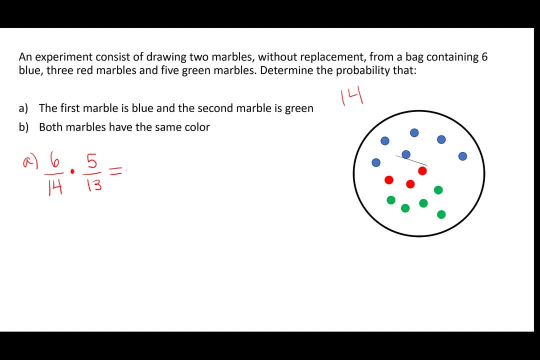 And so when you multiply these together- and please use your calculator- you have fifteen over ninety-one, which is approximately sixteen point five percent. Part B is the tricky part. It says both marbles have to be the same color. Now it doesn't say which color. 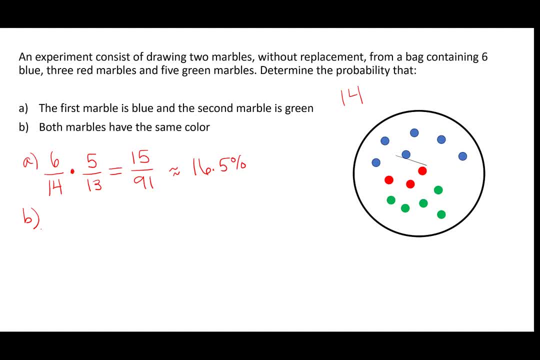 So we could pull out two blues, we could pull out two reds or two greens, And so I'm going to write that sentence that I just said, you know, as a probability statement. So we have the probability of BB, which means blue. 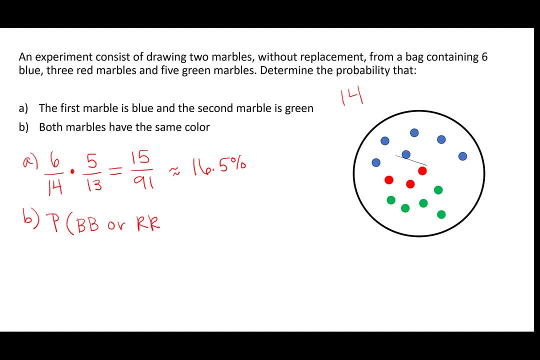 or RR, which is red, or GG, which is green. So what we're going to do is we're going to find the probability of each of these. Now, remember, we're not returning them the first marble back, So I'm going to write down the probabilities for each of these. 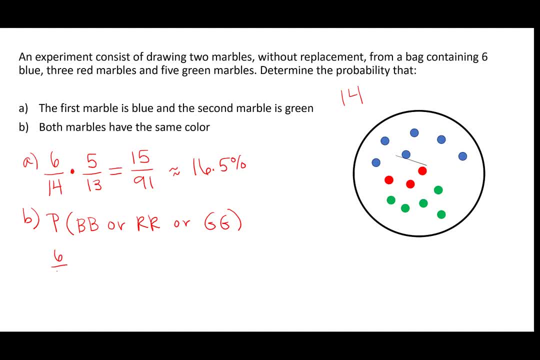 So for the blue blue, it's six over fourteen times five over thirteen. I'm going to just put that in parentheses. For the green- or sorry, I have red next, it would be three, fourteenths times two, thirteenths. 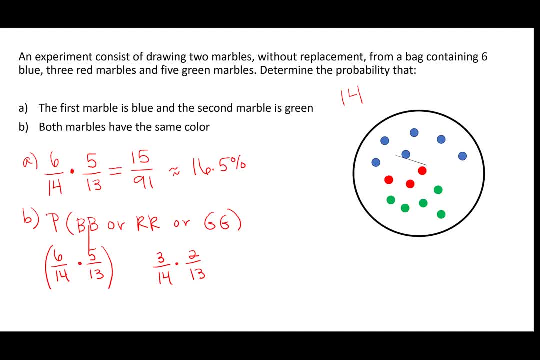 Again, the reason we're multiplying is because we're pulling out two items. We want blue and blue, Red and red. So I'm just going to put parentheses around those two fractions And then for green it's five out of fourteen times four out of thirteen. 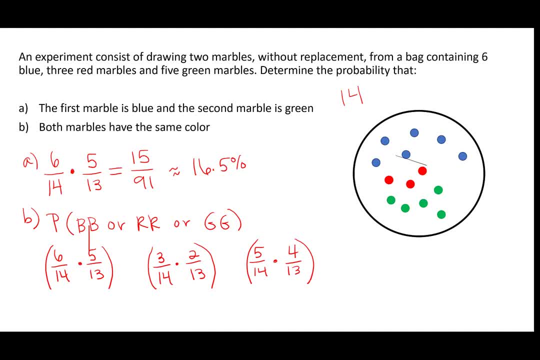 And again I'm going to put those. So I want to go back to the original problem. We don't need all of these to happen, We just need one of them to happen, One or the other or the other, And so when it's an or problem, 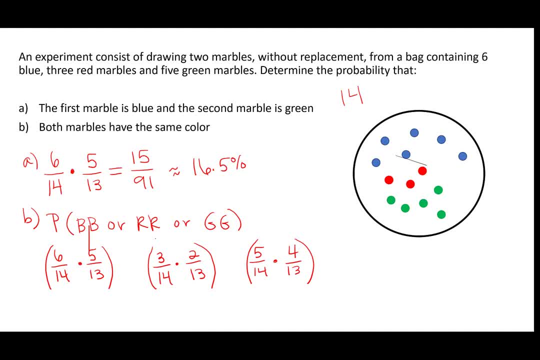 when you just want one of the selected items, that is an addition problem. So we are going to add what we put here in parentheses And this will just take some time to work through on your calculator. The blue blue when you add those together. 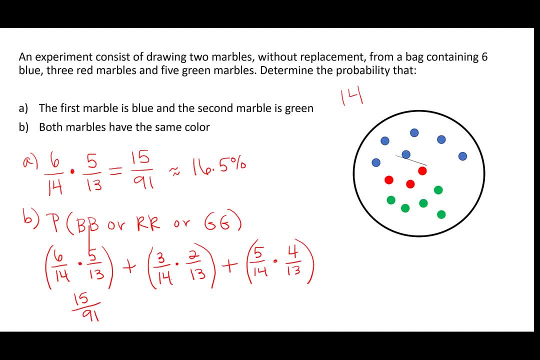 it's five over ninety-one. When you multiply the red- red, it's ten over ninety-one, And then the five fourteenths. the green green reduces down to three over ninety-one. Once you plug this into your calculator, you're going to get the fraction. 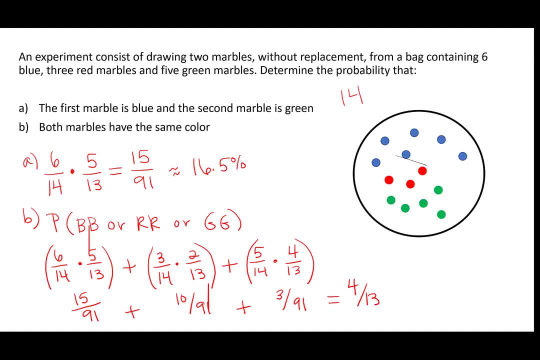 for thirteenths in most simplest form, which is about thirty point eight percent. So hopefully that helps. Message me if you have any more questions. Hi class, I wanted to show you this word problem because it could be a little tricky. 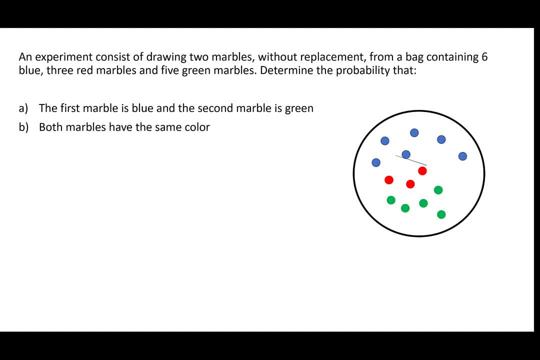 especially part B. Basically, we're going to be drawing two marbles without replacement, So the first thing that we need to do is count the number of marbles. Six plus three plus five is fourteen, And now we're ready to start the problem. 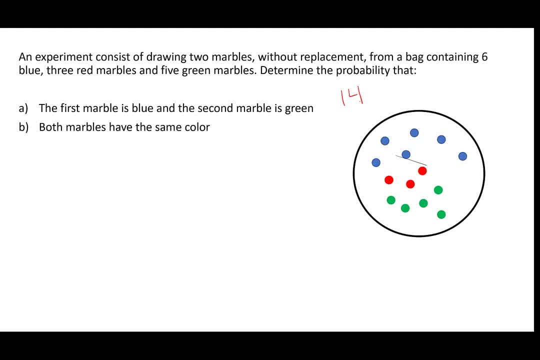 So part A is something you're probably familiar with from class. We want the first marble to be blue and the second to be green, In that order without replacement. So part A- the probability that it would be blue- is six fourteenths. 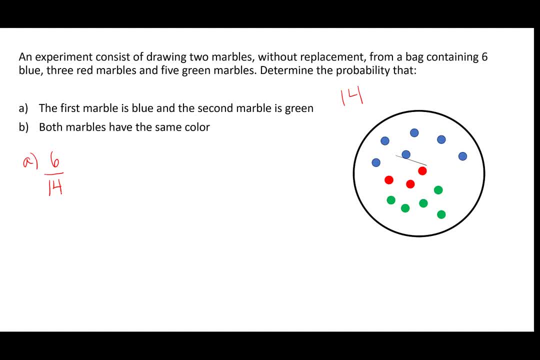 Then the probability that it would be green after one marble is removed is five thirteenths. And because we want both events to happen, we want blue and green and green. That's a multiplication problem, And so when you multiply these together, 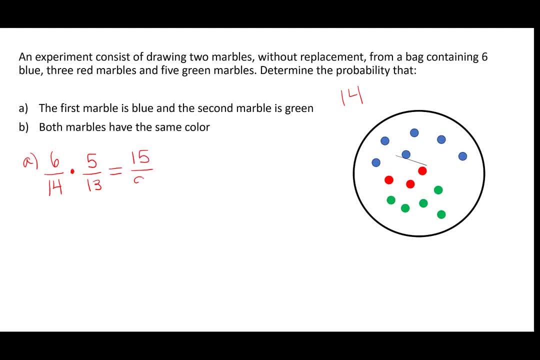 and please, you know, use your calculator. you have fifteen over ninety-one, which is approximately sixteen point five percent. Part B is the tricky part. It says both marbles have to be the same color. Now it doesn't say which color. 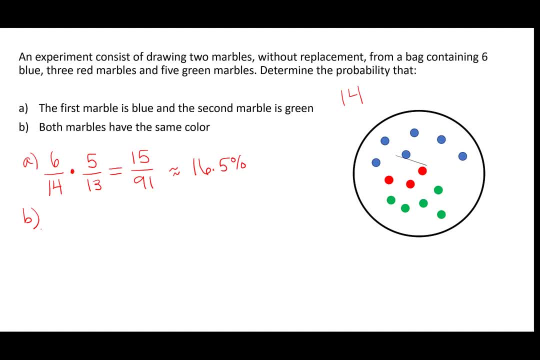 And so we could pull out two blues, we could pull out two reds or two greens, And so I'm going to write that sentence that I just said, you know, as a probability statement. So we have the probability of BB, which means blue. 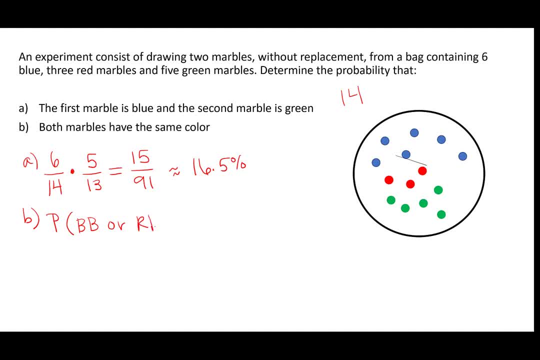 blue, or RR, which is red, or GG, which is green. So what we're going to do is we're going to find the probability of each of these. Now, remember, we're not returning them the first marble back, So I'm going to write down the probabilities for each of these. 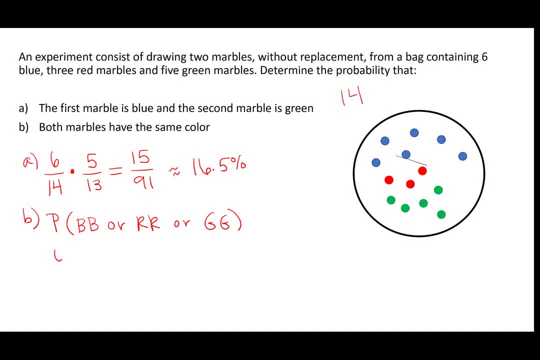 So for the blue blue, six over fourteen times five over thirteen. Okay, I'm going to just put that in parentheses. For the green- or sorry, I have red- next Be three fourteenths times two thirteenths. 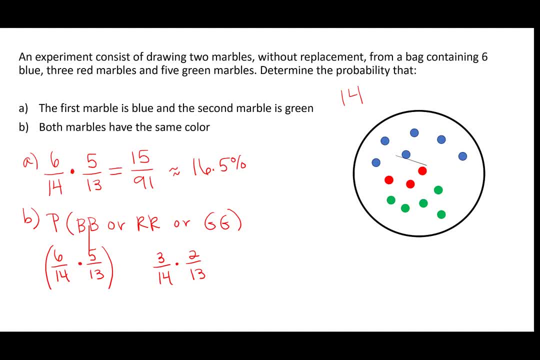 Again, the reason we're multiplying is because we're pulling out two items. We want blue and blue, red and red. So I'm just going to put parentheses around those two fractions And then for green it's five out of fourteen times four out of thirteen.